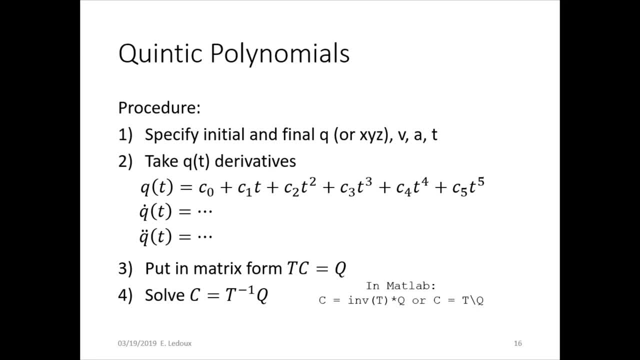 Q, double dot acceleration. then you put all of those in matrix form: T, C equals Q, where T is the time, C is the coefficients and Q is position velocity acceleration at start and end. So T will be a six by six, C will be a six by one, Q will be a six by one. 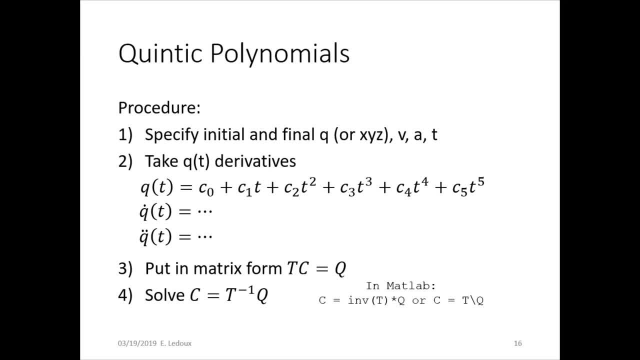 Then you can solve C equals T inverse Q using either the inverse function on a calculator, if your calculator does matrix inverses, or you can do it in MATLAB using the language shown. This is really difficult to do by hand, just because taking the inverse of a six by six matrix 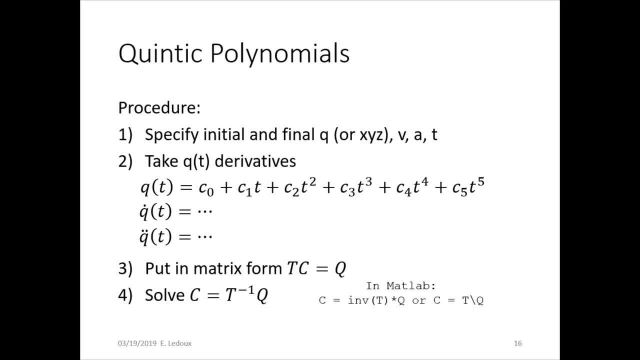 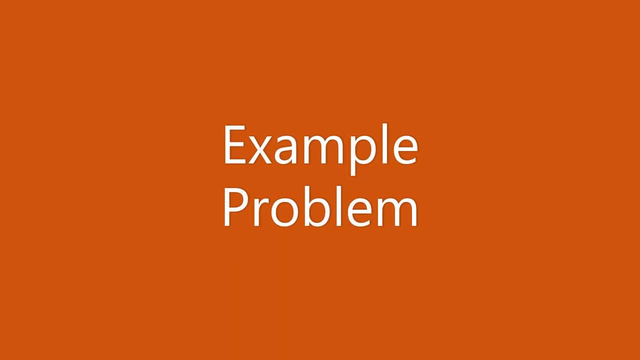 is kind of a monstrosity that you don't have to deal with, but you do need to be able to set it up completely and then just do the operation using a program or calculator. So let's do an example of this so that we can see how it works. If we're given that a robot joint moves, 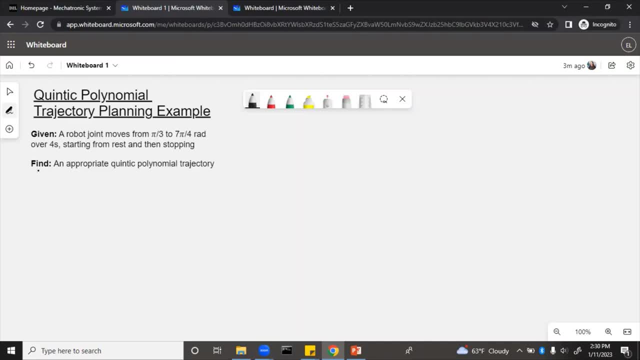 from pi over three to seven pi over four radians over a period of four seconds, starting from rest and then stopping, find an appropriate quintic polynomial trajectory. So what trajectory of a fifth order polynomial would make the robot joint move from the start angle to the end angle, starting and ending at rest over four seconds? 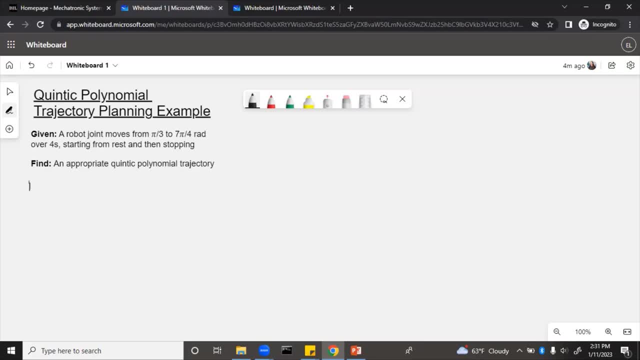 Well, first let's write down the procedure so that we can remind ourselves what order to do things in. Step one is to specify the boundary conditions. Step two is to take derivatives, Get velocity and acceleration. Step three is put in matrix form. 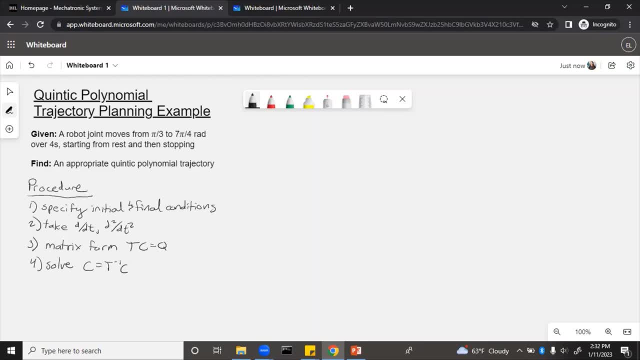 And finally solve. You can see the coefficients so that we can put those into the trajectory And up with the equation for Q. So step one is specify initial and final conditions. So let's make a table for that. We'll need to know initial and final position, velocity. 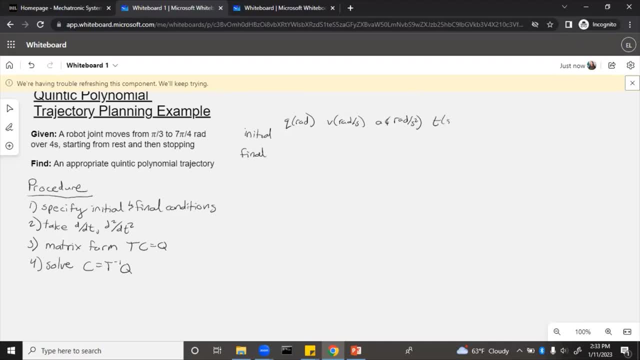 and time. So from pi over 3 to 7 pi over 4 radians. so pi over 3 would be the initial position and 7 pi over 4 is the final position. Then if it starts and stops, starts from rest and 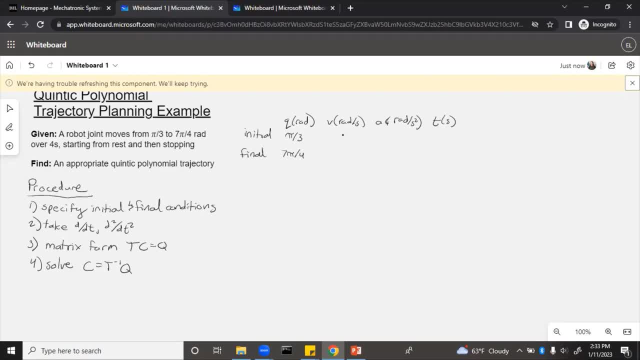 then stops. Initial and final velocity must be zero. Now velocity will not be zero during the whole trajectory, because that would mean the robot's not moving, But it starts from rest and then it speeds up and then it ends at rest. 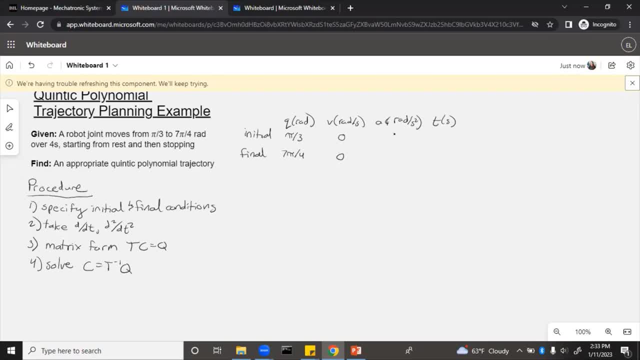 And so the acceleration would also have to initially be zero and be zero at the end, because the robot's not going to go anywhere after that. Then, finally, time: we assume that if it's a period of four seconds, say, it starts at time zero and ends at time four. 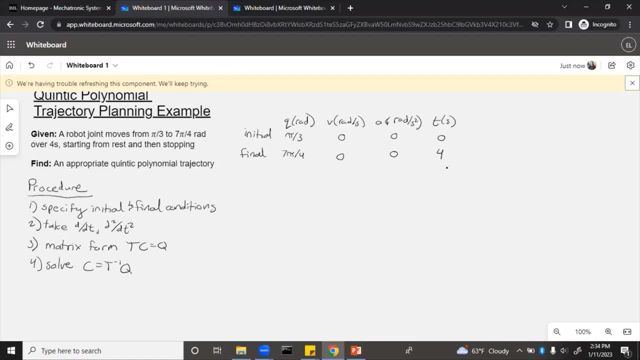 Now we have all of the parameters that we need. So next let's write the quinnipolynomial equation and then take its derivatives. So Q of t equals C0 plus C1 t plus C2 t squared, Plus C3 t cubed, plus C4 t to the fourth power, plus C5 t to the fifth power. 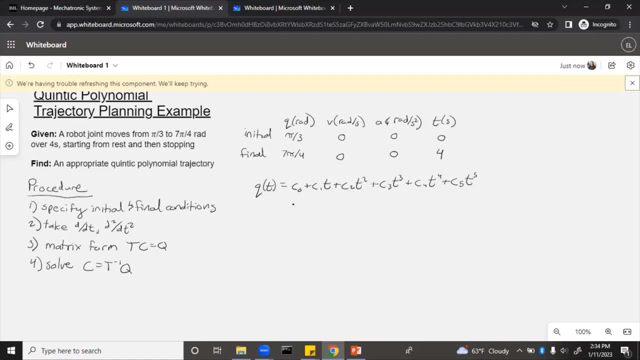 We don't know what those C's are yet, but we'll find them out. So then we take the derivatives to get velocity and acceleration. Next we need to put this in matrix form, So Will be T C Equals Q. 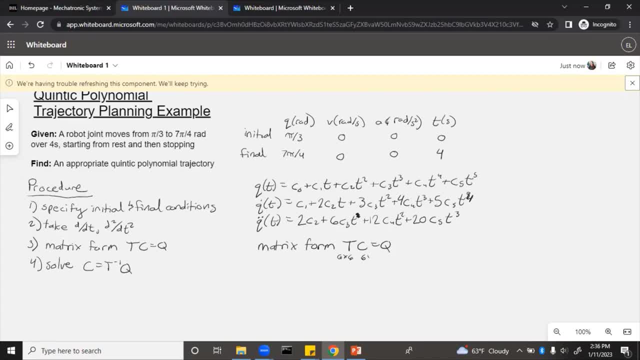 Where T is a six by six, C is a six by one and Q is a six by one matrix. So T will have T, We'll have the coefficients of the T variables in those equations And that will be multiplied by The C matrix, so that would be C0. 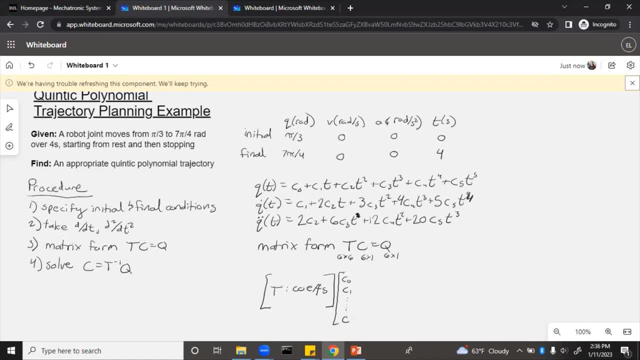 C1, dot, dot, dot all the way on to C5. And then that equals the Q matrix. so that will have Initial Position, velocity acceleration and then final. This is the basic form that it will take. 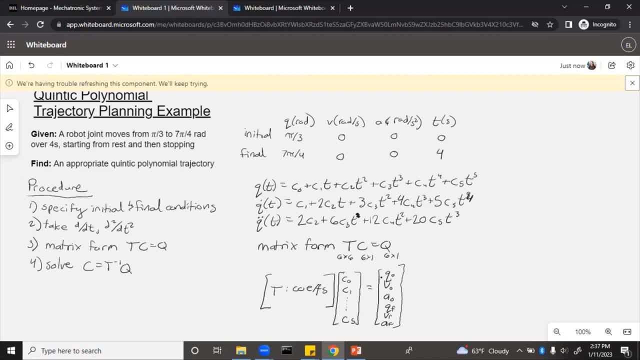 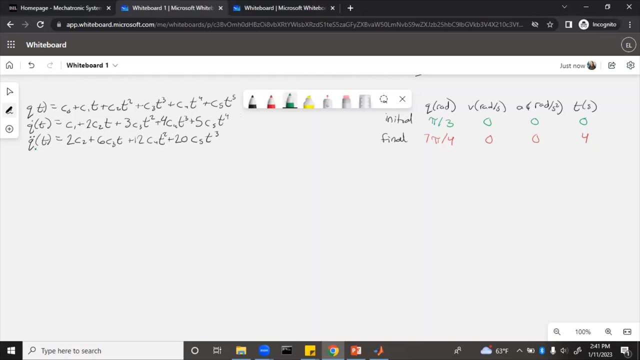 So In order to determine what numbers actually go in here, we need to plug in the initial and final values of T into these equations for Q Q dot and Q double dot. then we can put those into matrices. In order to put these polynomials into matrix form, we need to figure out what their actual values are at the start and the end. 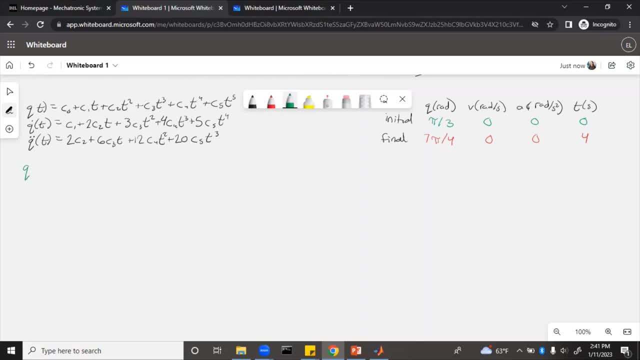 So If we Do Do Q of T At the initial, we just need to plug in zero for T. So if all the T's are zero, then basically this just equals C0.. Now for Q dot Similarly, this would just equal C1.. 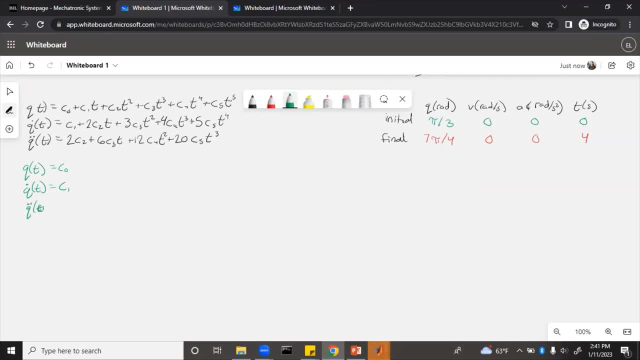 And Q double dot At zero is going to equal to C2.. Now the ending one is obviously going to be more complicated. so we plug in 4, q of 4, and then q dot of 4, and then finally q double dot of 4.. 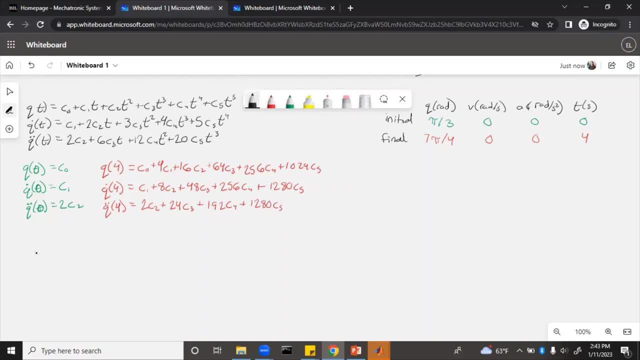 Now we have all of the equations that we need to be able to fill out a matrix. So let's make a 6x6 matrix. So let's make a 6x6 matrix for the coefficients of c. So basically, everything that's multiplied by a, c, in these equations will go in that. 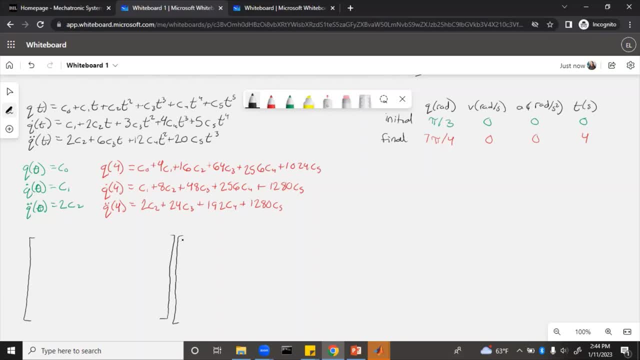 big first matrix and then we'll put all the c's here in the second one, So c0, c1, c2, c3, c4, c5.. And then this is going to equal q0.. v0, a0, q, final, v final, a final. 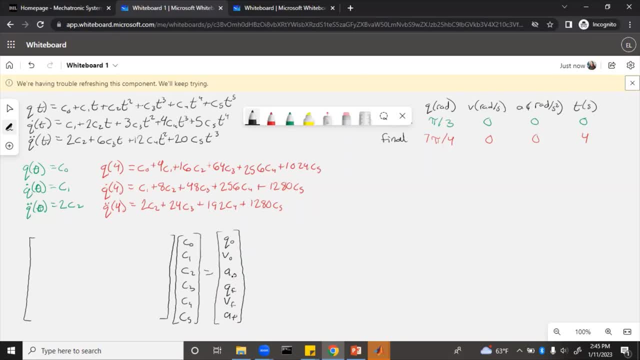 Now, all of these q, b and a- initial and final- were given in the problem statement, So we can actually just replace all of those. The initial, we had pi over 3. 0, 0.. And then the final, we had 7 pi over 4, 0, 0. 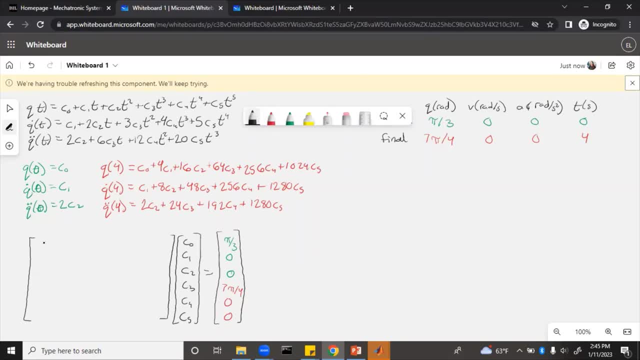 So now, in order to fill out this T matrix, we need to figure out what goes in all 36 of those locations. So each row is gorgeous And each column is going to correspond to the q, v or a. So this all corresponds to q0, v0, a0, qf, vf, af. 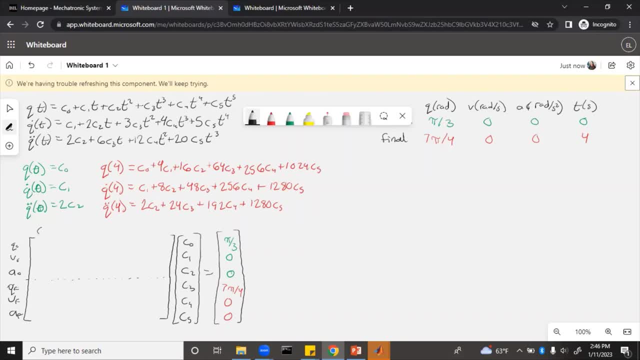 And then each column corresponds to the c- c0, c1,, c2,, c3,, c4.. And then each column corresponds to the c- c0,, c1,, c2,, c3,, c4.. And then each row corresponds to q0.. 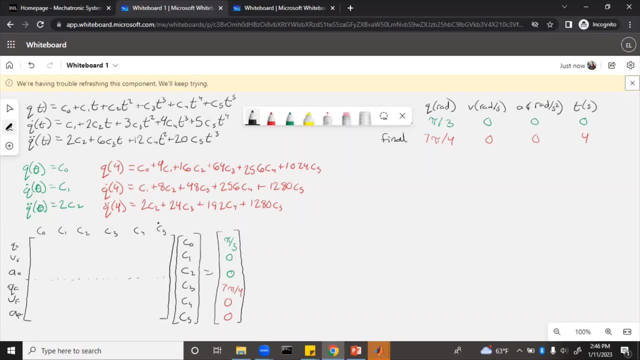 v0, a0, qf, vf, af, C4, C5.. So now we just need to fill those out. So for the Q0 equation, whatever is multiplied by C0 would go in the first spot, and then whatever is multiplied by C1 in the second spot, and so on. 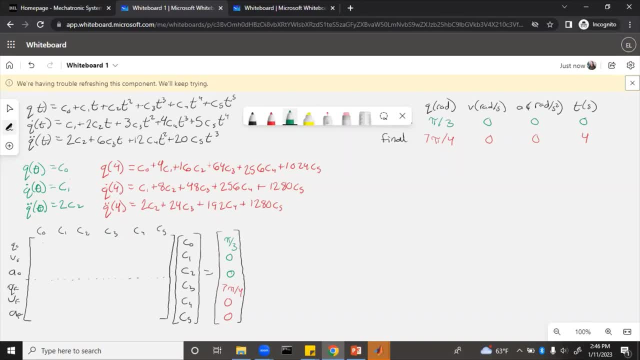 Well, Q of 0 is just C0, so that coefficient is 1.. There's one C0 there. Everything else is zeros. Now, initial velocity, Q dot of 0, is just C1.. So we have a 1 in the C1 spot and we have zeros everywhere else. 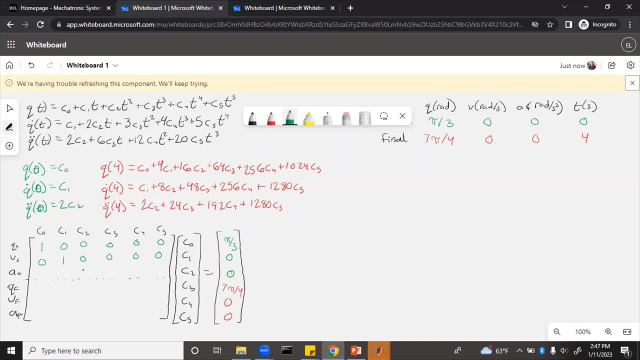 Then Q double dot of 0 is just 2C2.. So we'll have a 2 in the C2 column and zeros everywhere else. Now the final one is obviously trickier, but all the coefficients are easily visible. So C1, there's just one of those. 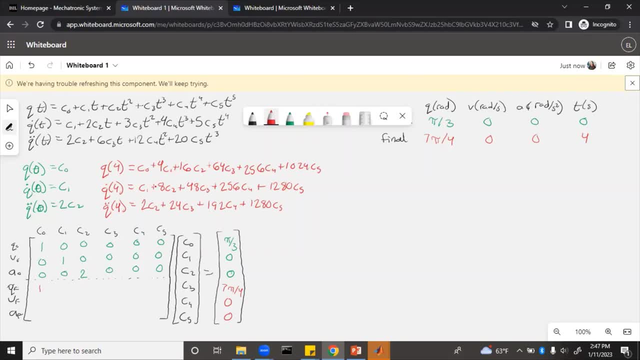 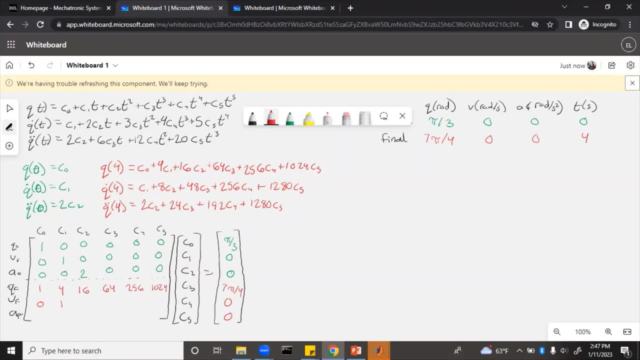 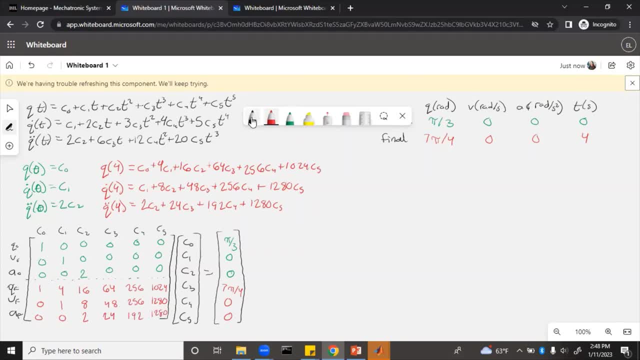 So now that we have these filled out, we'll write the form up here: T times C equals Q. We need to solve this and figure out what those coefficients are. C equals T inverse Q. So you can do that on a calculator or you can do it in MATLAB. 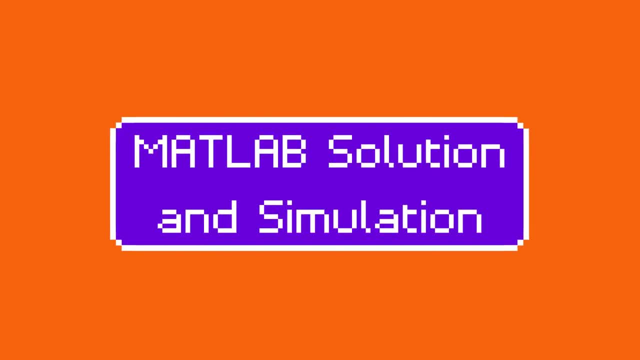 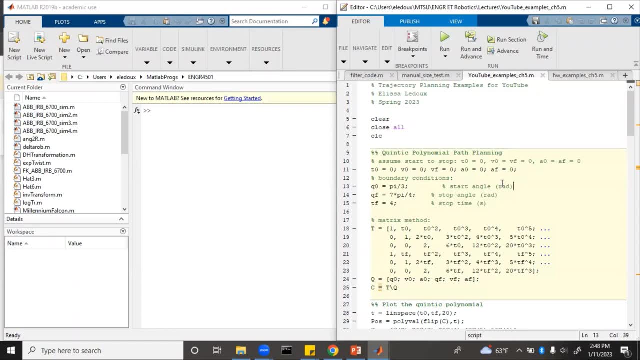 So let's look at MATLAB. So here you can see I have input, all of the boundary conditions as well as the time filled out the matrices, and then write the equation. So we run it And we get the C matrix right here. 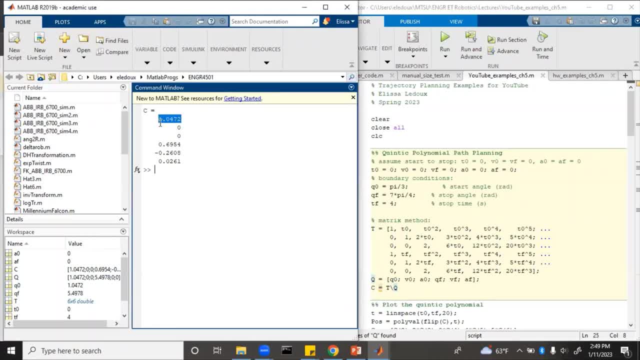 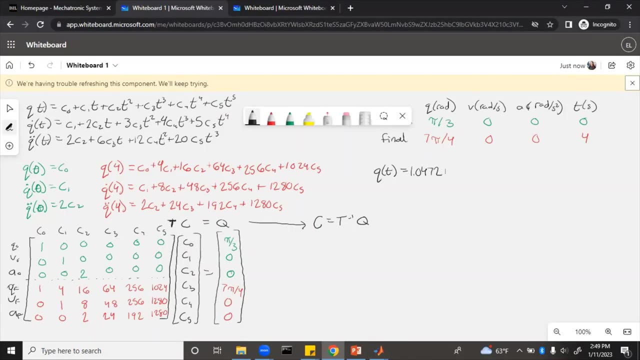 So this is the coefficient, or that's what C0 equals, And then C1,, C2,, C3,, C4, and C5.. So those are the coefficients that would go into the polynomial trajectory. So this is the answer for the quintic polynomial trajectory. 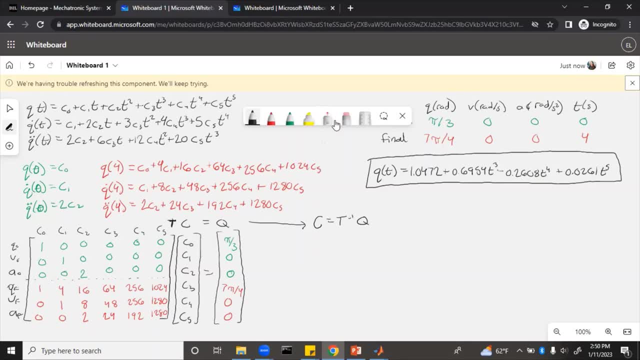 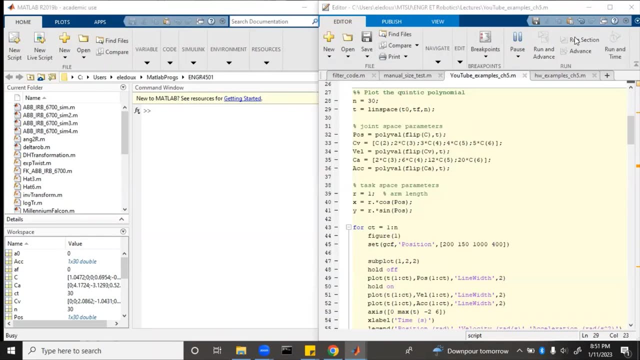 There's a chance that you can get something that's as far from C aserez, So you can get this first, But there's no way you can get really the second time with the definition because you have to actually write ourremlin. We're going to think about things from the E left side. 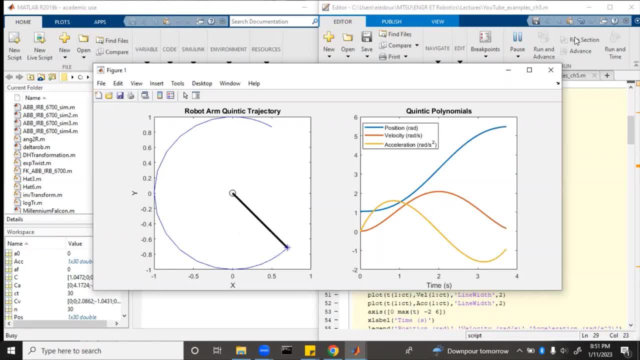 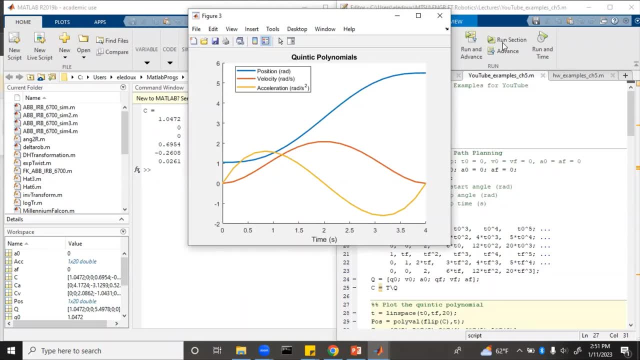 So let's look at the things from the E right side. We're going to set up aoriented to the a is the price of our polynomial. We're going to come in here and say I am just going to apply the Joker At any price range of $17.. 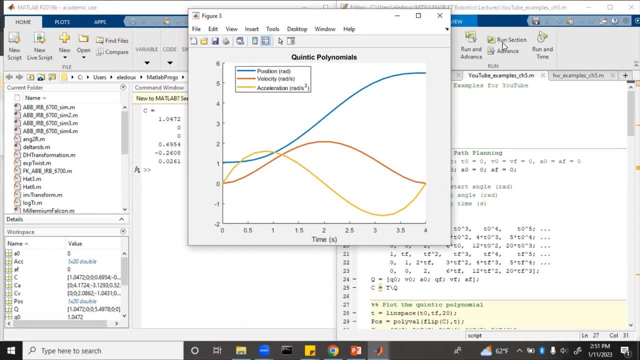 And we should Noch ярftx, so you could say mcs. And here's a opardx. What's up? position being a quintet polynomial, and then velocity being a fourth order, acceleration being a third order, And then, if we verify the boundary conditions, time on the x-axis here goes from zero. 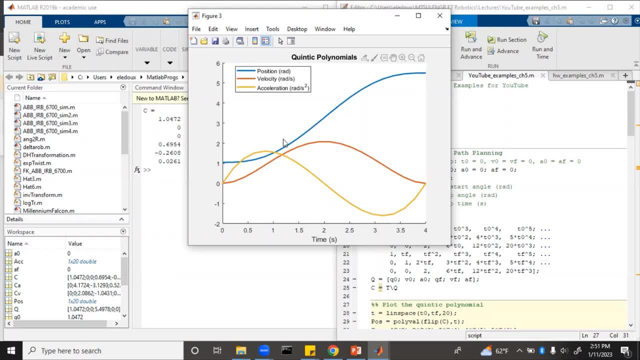 to four seconds. That is correct. Position goes from a little bit over one, which is pi over three is close to one, up to five and a half, which is basically seven pi over three. And then you can see that velocity and acceleration both start at zero and end at zero, but are not zero the whole. 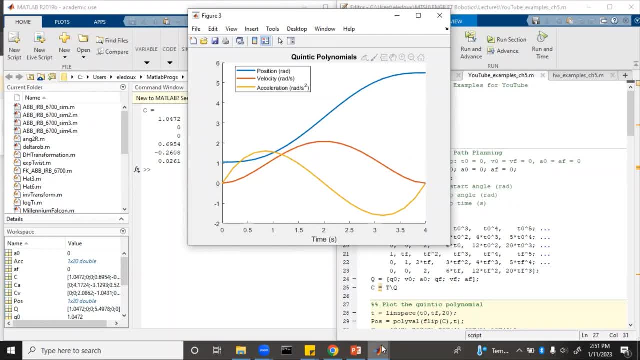 time. So this passes the reality check. C1 and C2 both ended up to be zero. This is actually always going to be the case if initial velocity and acceleration and final velocity and acceleration are both zero. So if you have final and initial velocity and acceleration both being zero, 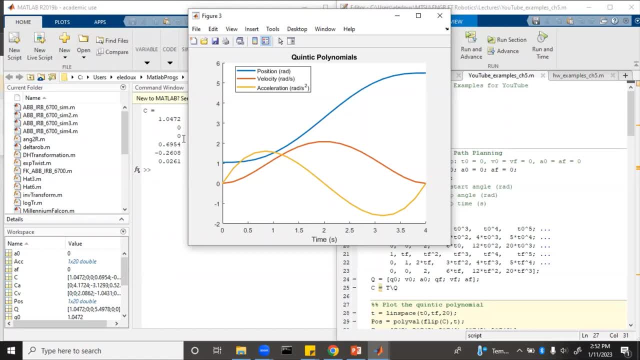 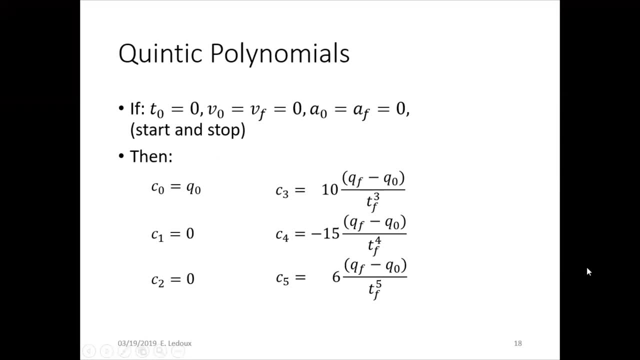 then C1 and C2 will always be zero. There are also some shortcut formulas that can be solved by hand for this special case, So these formulas are what you can use to solve the special case of zero velocity and acceleration at the beginning and the end.